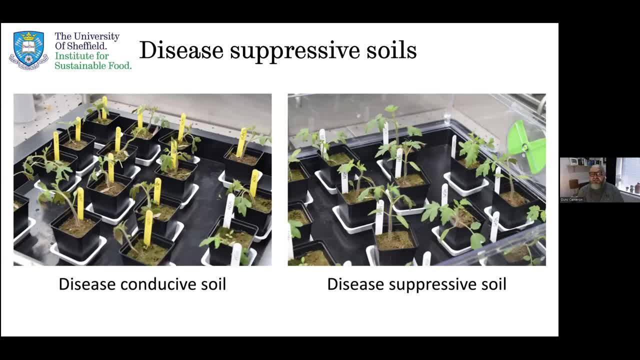 The soil type is the same, the nutrients are the same, yet if you infect the plants with a foliar pathogen, as we've done it to both of these sets of plants, you can see the plants that grow in a disease conducive soil have been obliterated by the pathogen and that's in. 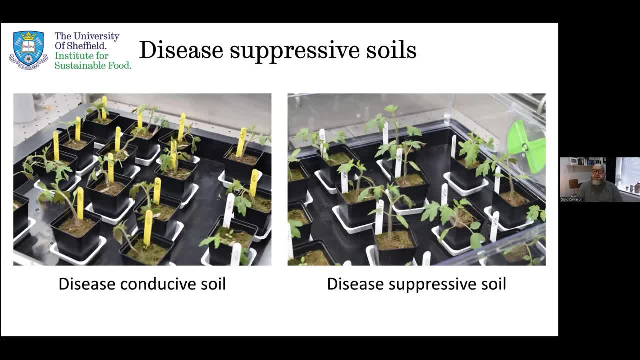 just 48 hours, But when we have a look at the plants that are growing in a disease suppressive soil, we can see that there are no to little signs of that foliar pathogen destroying its host plant, which I think is really phenomenal. and 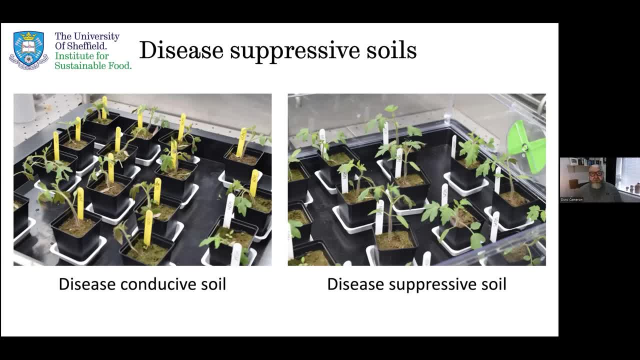 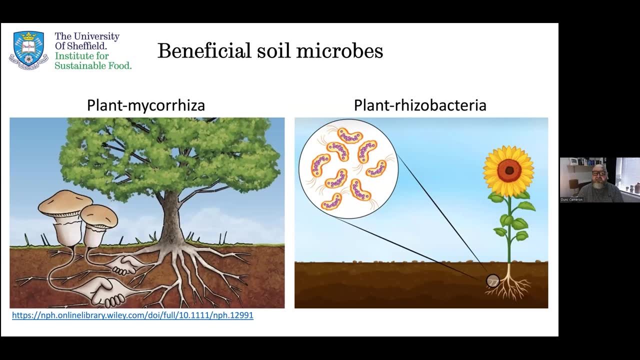 I think it offers some real opportunities, if we can understand it, to begin to control diseases without the use of pesticides. And there are a range of symbiotic, mutualistic symbioses in the soil. I think a lot of you will be familiar with the idea of mycorrhizae. so these are symbioses between: uh 95 percent of all plants and uh four percent of our plants as well. Of course, these are not reagents, so it's aаш. in other words, we are simply organic. If we have some bacterial host plant, we are wanting to find things like hypo growth. 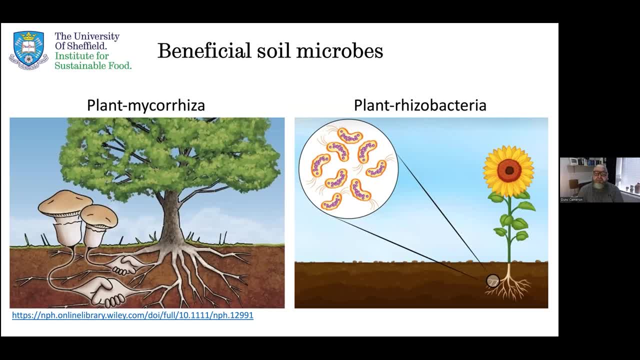 reptiles, gr Programs. They begin to change because of these bond with a airports without pesticide effects, plants and soil-borne fungi, and here the plant supplies the fungus with carbon in return for nutrients. and that's what we kind of thought the symbiosis did. that's the full extent. 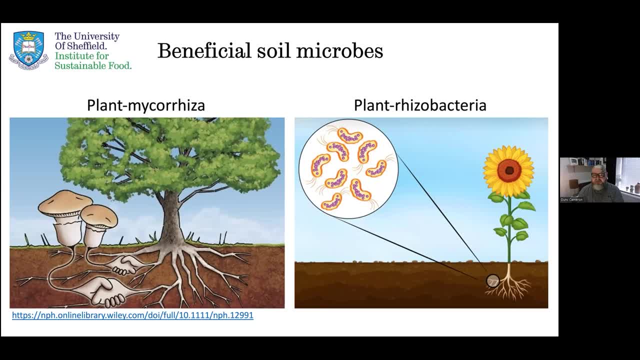 of it and hopefully I'll convince you later that there is something much greater and possibly more interesting to this symbiosis. But we also have bacteria in the soil that associate with plant roots, and many tens of thousands of bacterial species occupying the zone around a plant root that we call the rhizosphere. Now, the rhizosphere is the area of the soil. 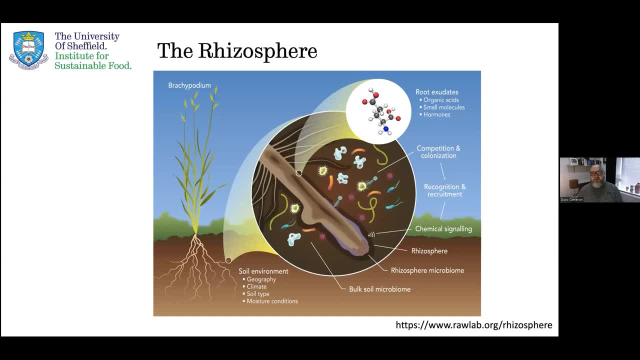 around a plant root that is in direct chemical control of that plant. so plants exude lots of compounds through their roots into the soil that have a range of different purposes, and the extent of the limit of these compounds to influence the soil is called the rhizosphere, or that's at least one definition and my definition of the rhizosphere. 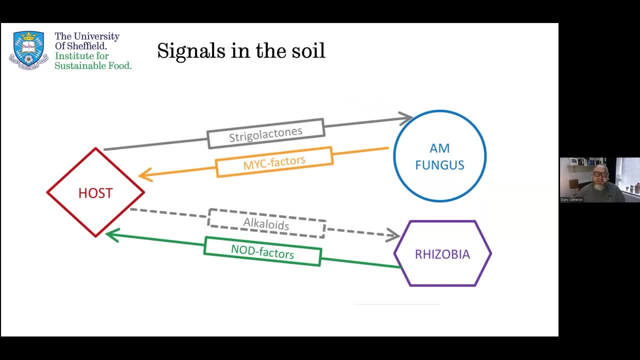 Now, within the rhizosphere, we can kind of think about it almost as an information superhighway. A plant, which is here represented as the diamond Oh, signals out to attract fungi and different types of bacteria and they can respond to the plant and change how the plant's physiology, the plant's functioning is, is regulated. 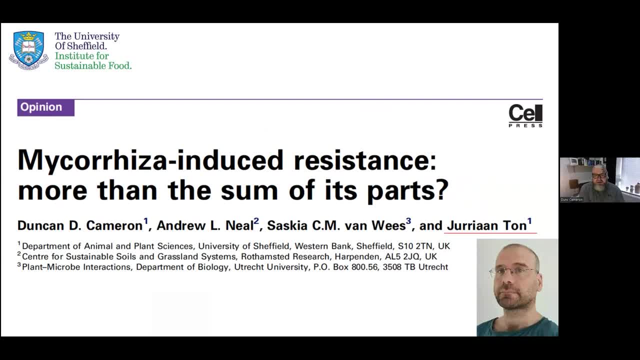 and a number of years ago, a colleague, a long-term collaborator of mine and I, Urien Ton, came up with an idea about how these different types of organisms within the rhizosphere could influence plant health, and we built a mechanistic model that is simplified here and, if you're interested, 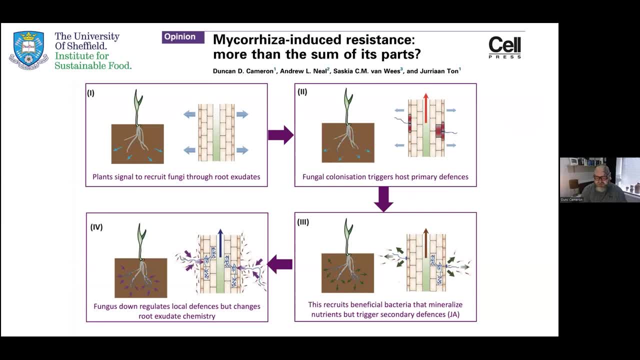 this. this publication provides more detail where, essentially, plants send signals out into the soil and they want to recruit things like fungi that can come along, and when they interact with the plant, they they are going to trigger the plant's immune system. plants have an adaptive immune system that allows them to deal with pathogens. 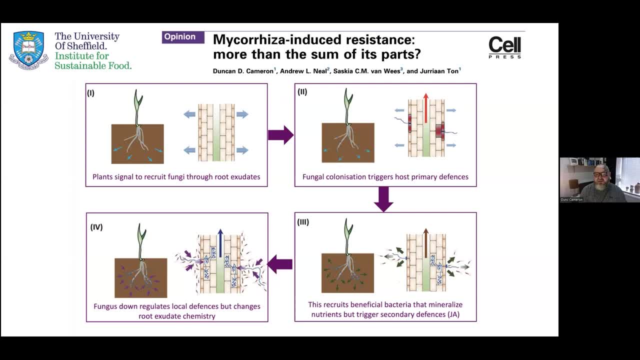 and here these fungi will trigger these plant defenses. but of course, if you're a symbiont, you don't want those defenses to kill you. what you want is to be able to tell the plant you're friendly and turn off those defenses, which is exactly what what mycorrhizal fungi can do. they can produce. 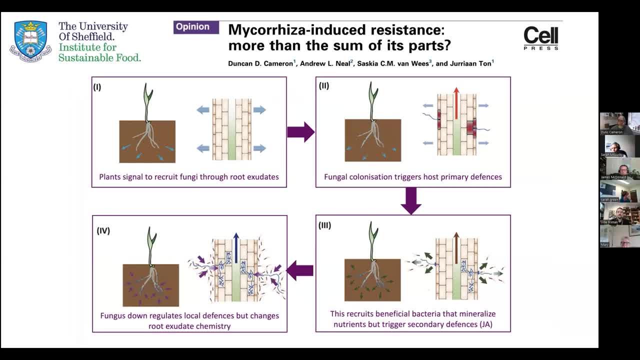 what we call effectors that tell the plant's immune system to calm down, but not before the plant has sent a signal above ground to warn it's above ground tissues that it might be being attacked and to ready themselves for defense. in the process, then, of sending these signals, the to the to the fungus, the mycorrhizal fungus, it. 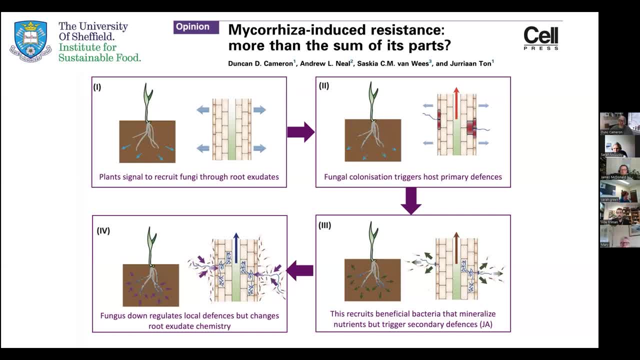 influences the chemistry of the exudates that are produced by the plant, and we we know that in some cases there have been observations that mycorrhizal fungi can cause the recruitment of beneficial bacteria into uh, into the, the rhizosphere uh, and they in turn can influence the host plant's. 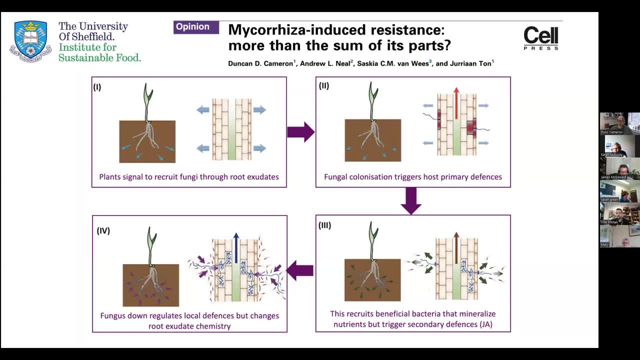 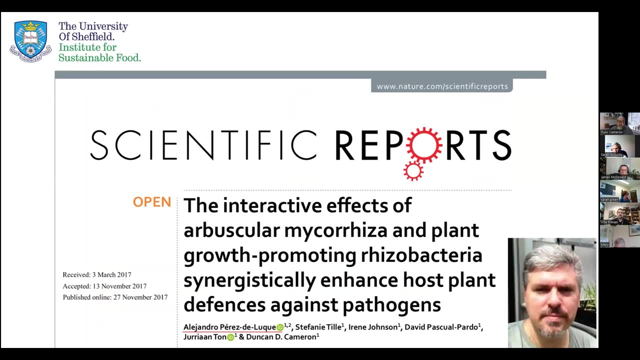 defenses. so we have this multimodal mechanism of how the plant is essentially outsourced much of the regulation of its immune system to the organisms that live in its rhizosphere, and we were able to test this model a few years ago, um, and we were able to demonstrate strikingly that 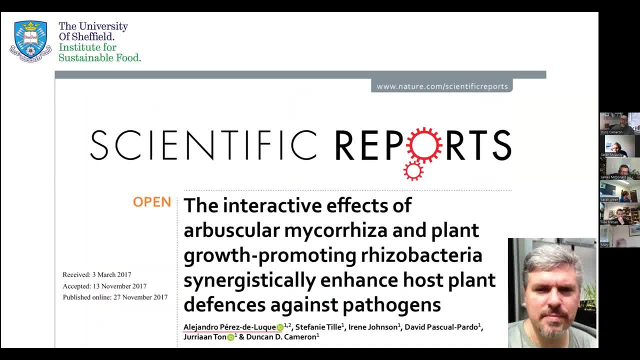 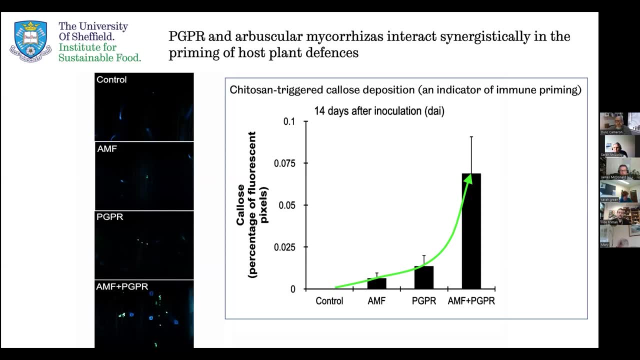 the host plant's defenses and their immune systems. uh can restructure the, the communities of um of beneficial bacteria that live in in the rhizosphere, and they can also impact on plant health. so here we've got a simple graph um where we had artificially triggered the host plant's 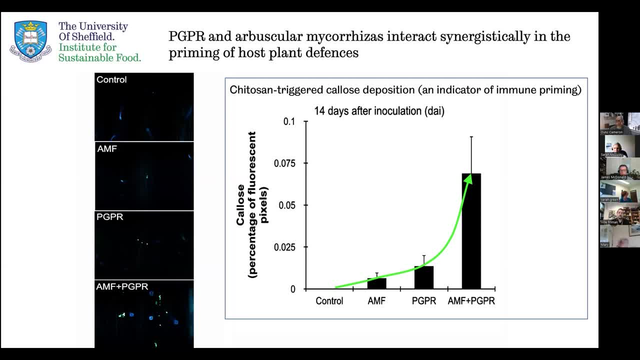 defenses um the the strength of their response depends on how activated or how primed their by bacteria and fungi in the rhizosphere. and, as you can see, if AMF means mycorrhiza, PGPR means plant growth promoting rhizobacterium, and when you add them together, the induction of 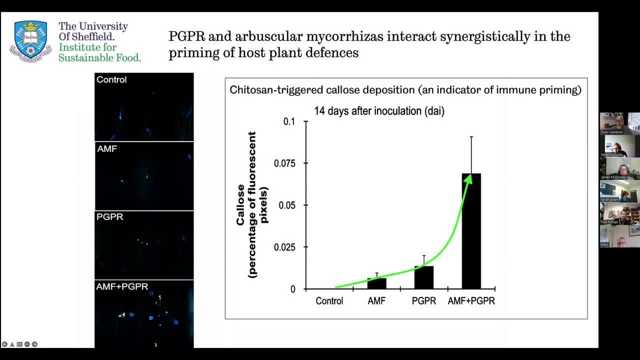 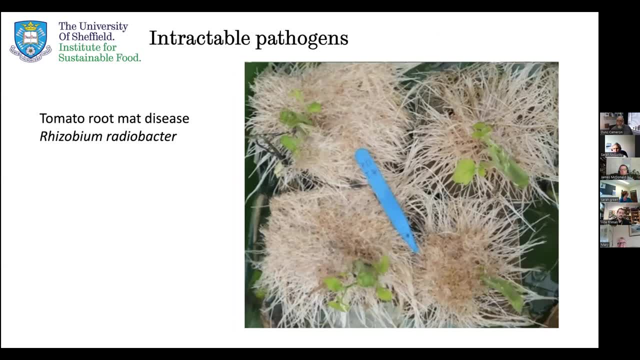 defence is synergistic, so having more of these organisms in your rhizosphere is a good thing. So just in the last three minutes of my talk, I'm going to talk about the pathogen that we work on. it's called tomato root mat disease or rhizobium radiobacter, and it causes these absolutely. 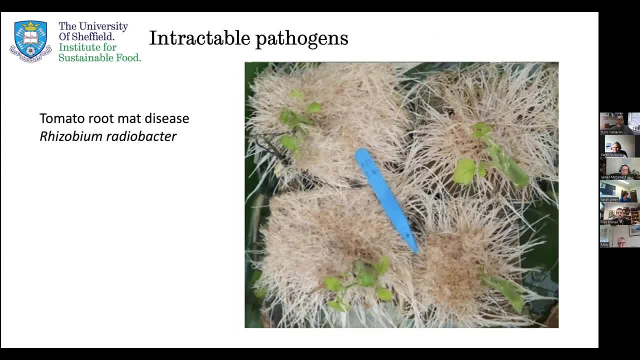 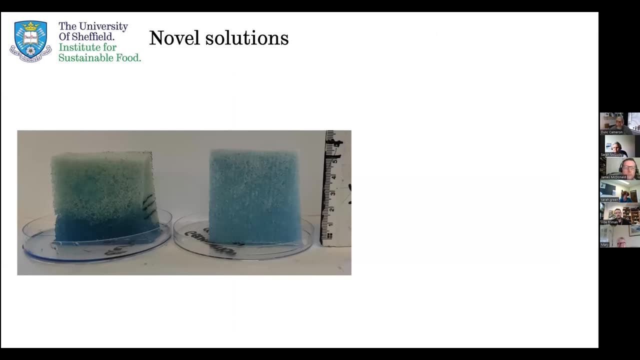 ridiculous protrusions, proliferations of roots in their host plants, which are tomatoes, and essentially this means all of the carbon is used to grow roots and there's nothing left for shoots and fruits. and one of the big issues is that this problem is intractable. there's no chemical control. 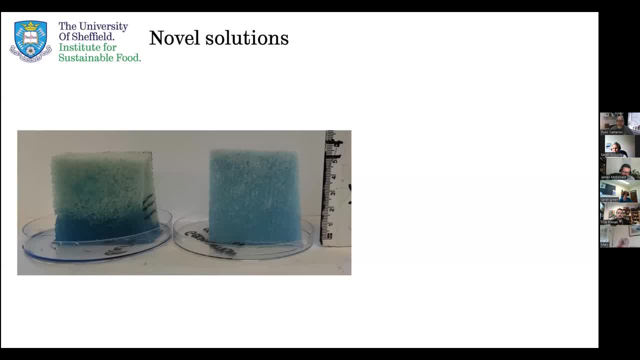 and when it gets into a greenhouse, because most of our tomatoes are grown through hydroponics. in a greenhouse, it runs riot. So what we've proposed is a novel solution, is doing away with the traditional substrates that you use in hydroponics, which is things like: 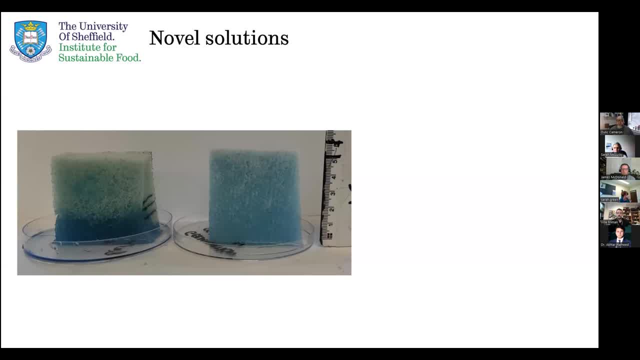 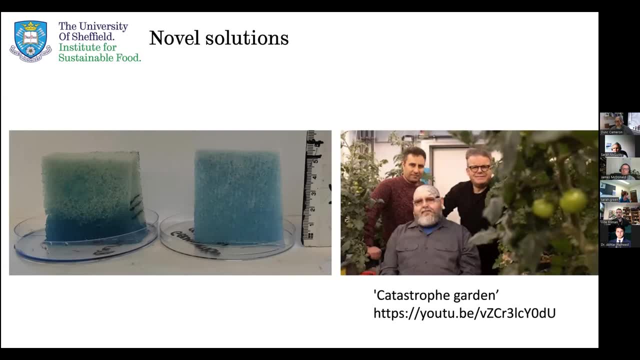 wool or coir matting and actually engineering a substrate which is designed to take advantage of beneficial bacteria and, if you're interested in growing plants in foam, in this case old mattresses. a quick plug for the recent documentary that we have made about our work, called the catastrophe. 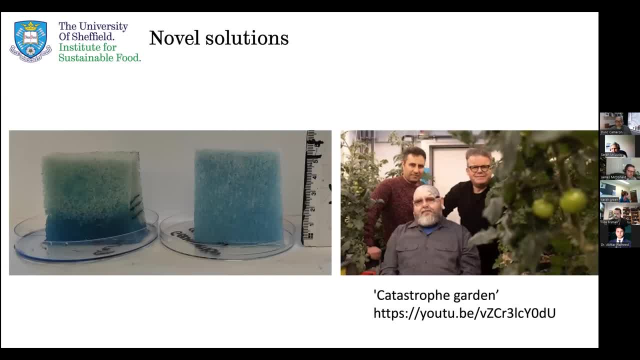 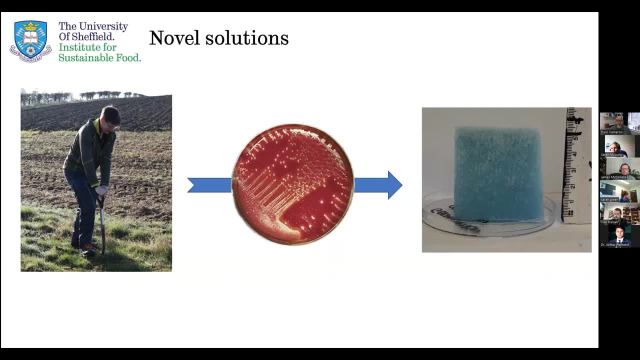 garden where we've grown food in a refugee camp in Jordan, with Syrian refugees using old mattresses. So our novel solution is to look to the environment, look to these disease suppressive soils in the way, in the kind of way that James has mentioned, to harness and isolate those bacteria. 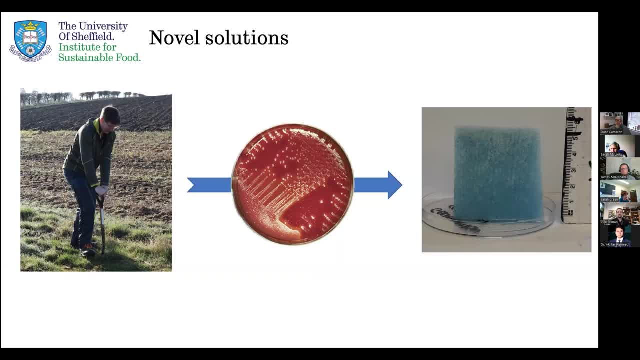 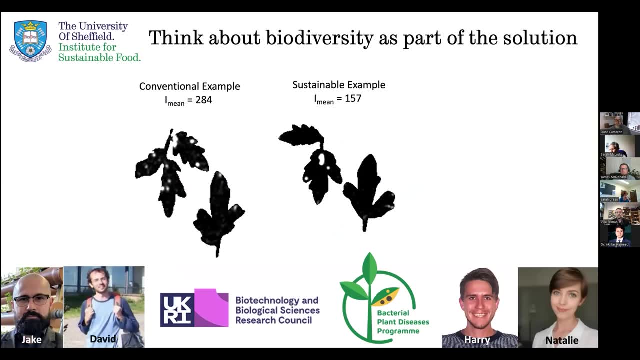 and then to assemble communities within artificial substrates that suppress disease, and we've been able to get quite a long way in terms of doing that. what we've done is to to harness a bacterial pathogen that attacks the roots as a a sentinel, as a an indication of 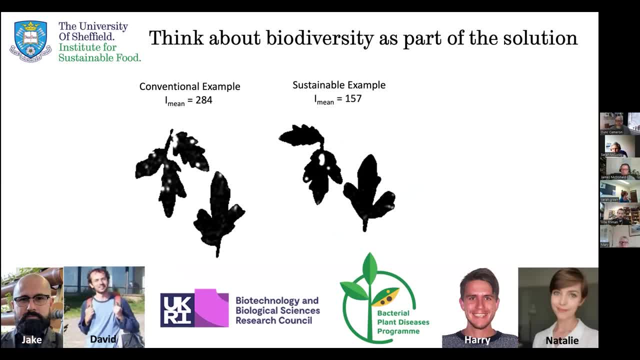 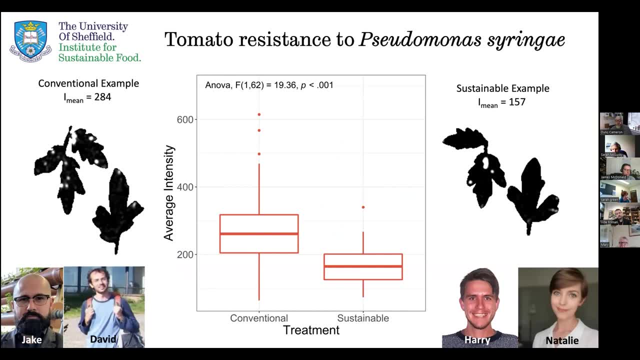 that this immune system is activated and we've made these, these bugs, glow so we can see them. and we've been able to have a look in different types of soils. we've got a disease conducive soil, which is the the left hand bar and the right hand bar. 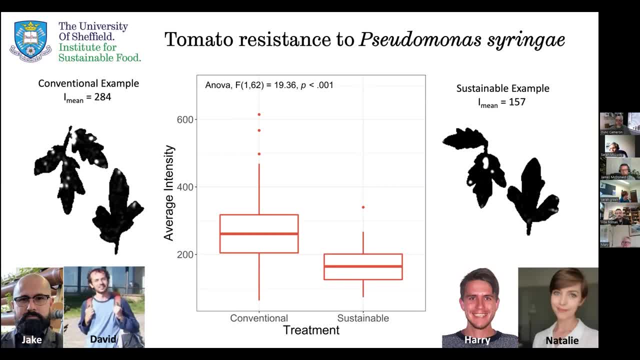 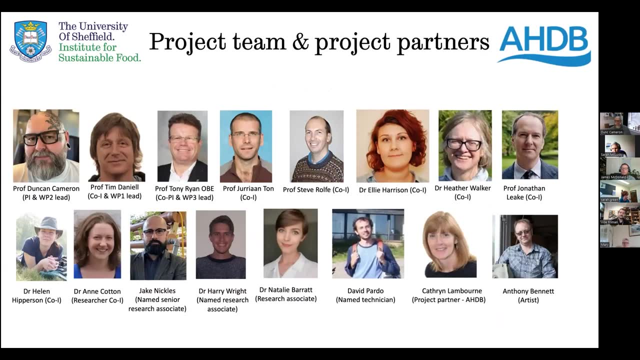 is a disease suppressive soil and we've really shown that the disease suppressive soils can suppress the pathogen. but also we can transfer the the microbial communities from the wild into synthetic substrates and they still suppress the pathogen. Now I think that's my time. obviously these projects are huge and it's impossible to. 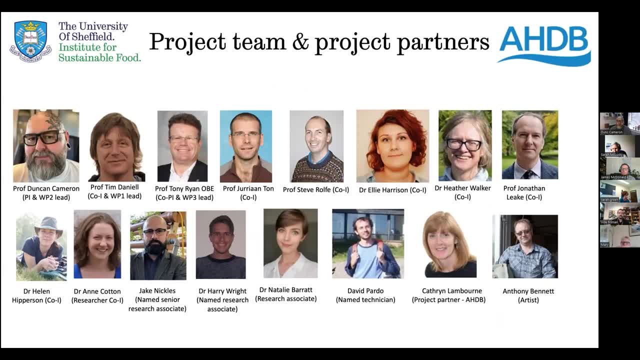 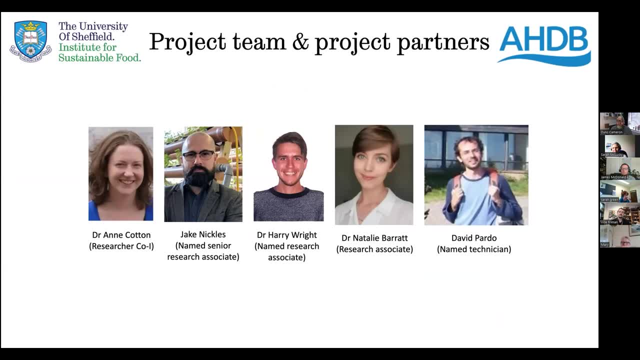 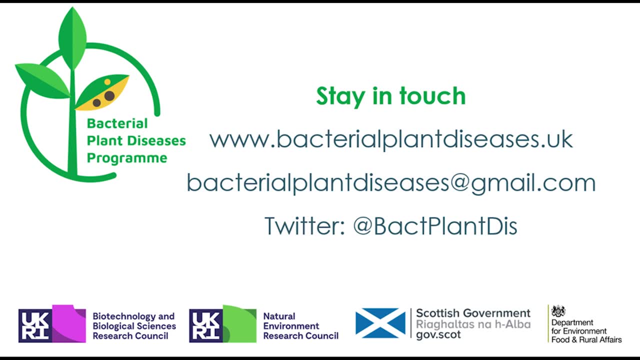 say what everybody has done, but this is what the team looks like. but I think what I really need to do is acknowledge the important people in the team. they're the postdocs and technician who've actually done the hard work. thank you very much. Thank you.